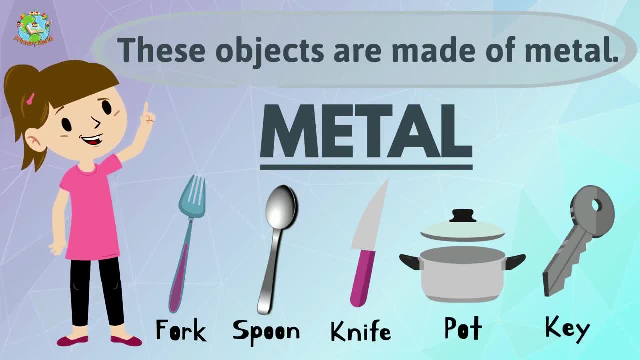 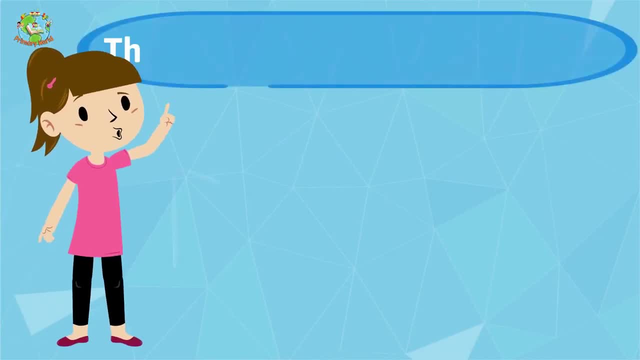 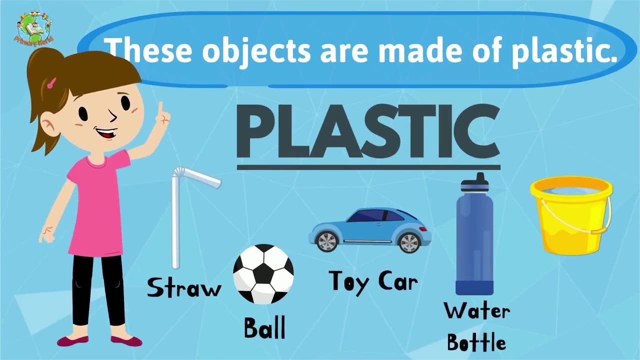 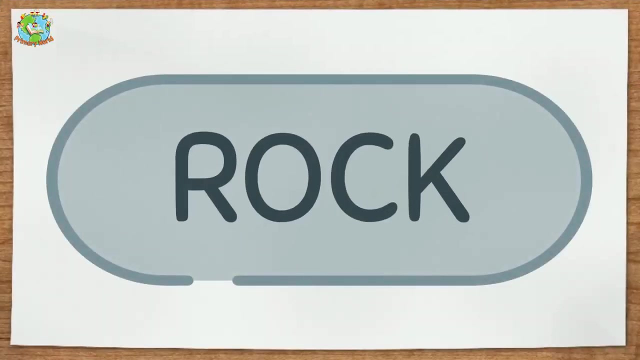 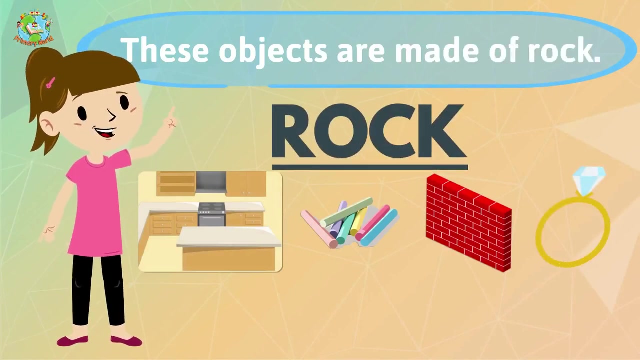 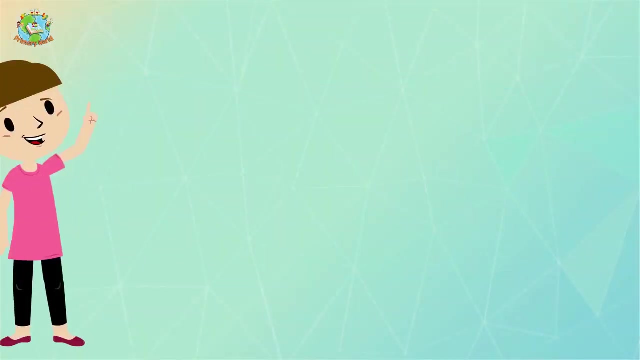 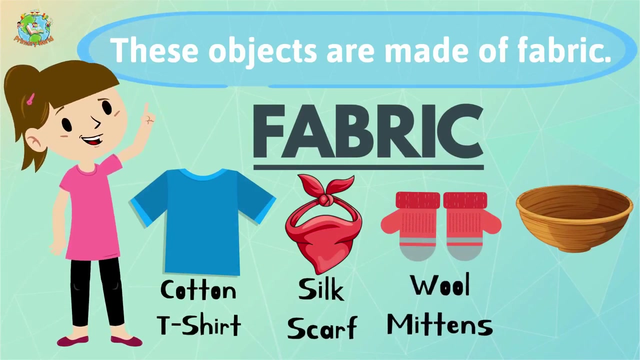 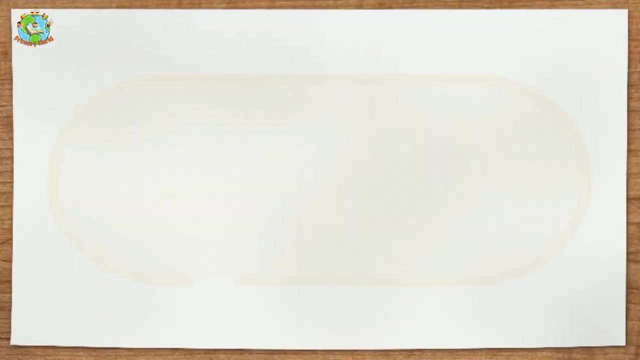 Plastic. These objects are made of plastic: Straw, ball, toy, car, water bottle, bucket, Rock. These objects are made of rock: Kitchen worktop, chalk, wall, diamond, ring. Fabric. These objects are made of fabric: Cotton, t-shirt, silk, scarf, wool, mittens, bamboo, ball, rubber. 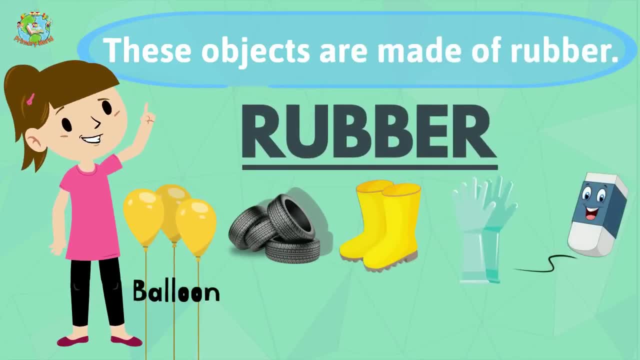 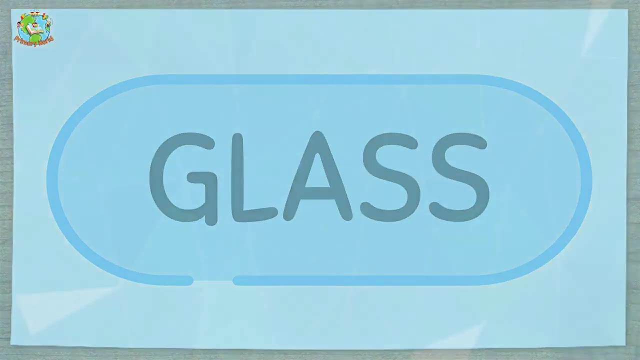 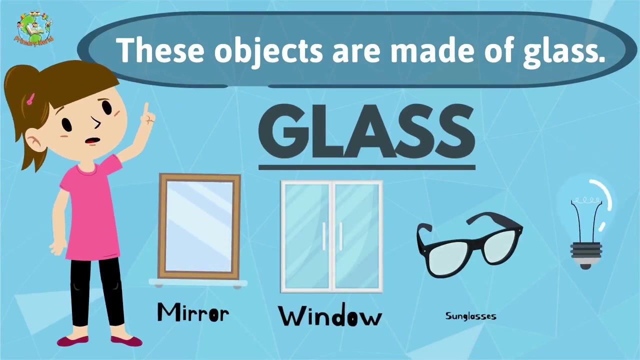 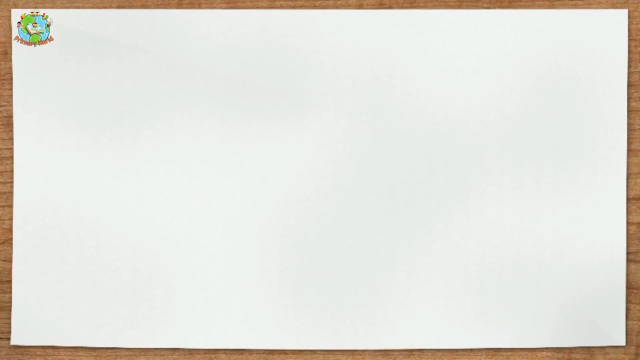 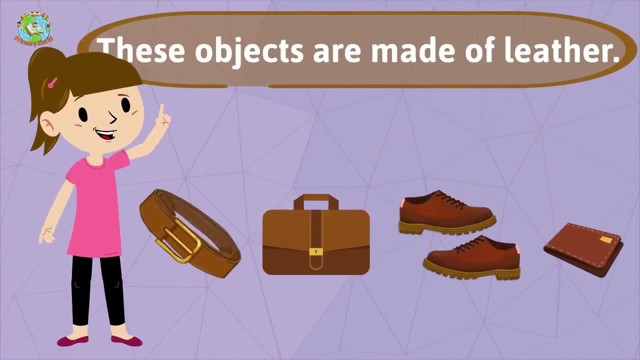 These objects are made of rubber, Balloon tyre, rubber boots, latex, gloves, rubber, Mirror glass. These objects are made of glass: Mirror window sunglasses, light bulb, Leather. These objects are made of leather: Belt, bag, shoes, wallet.